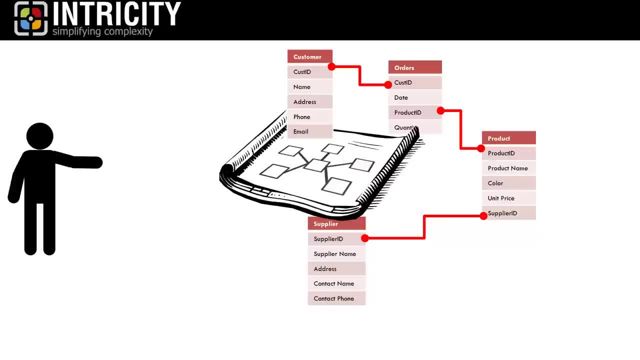 the relationships are within a database. This framework, in the world of data warehousing, is a critical component, as it will provide the structure which will support the analytical needs of the decision makers. The data itself will literally be stored within this framework on a database. So building a data model is a critical step in the design of a data warehouse. 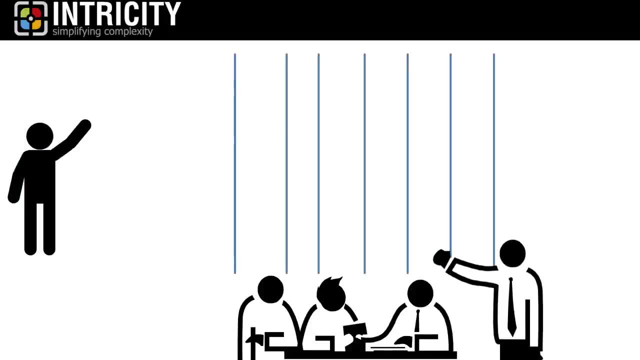 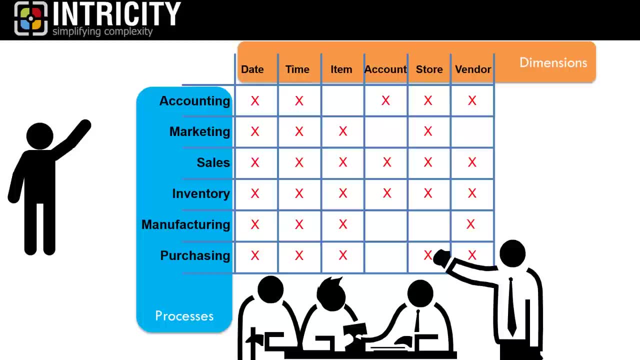 This step requires your business people to engage in the process by participating in facilitated sessions with our data architects. This can seem intimidating for organizations to take on so often they start looking for something out of the box. But here's the kicker that most people 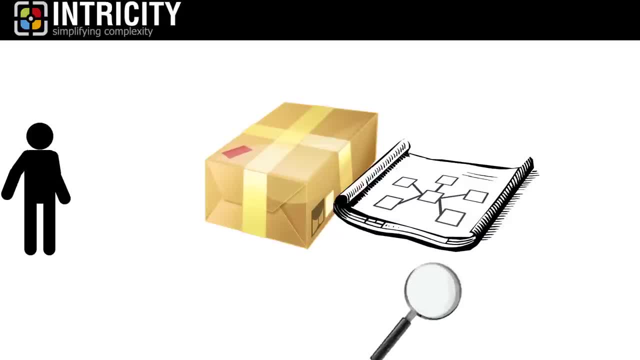 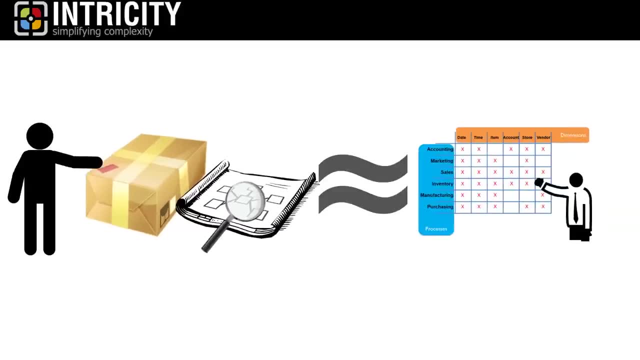 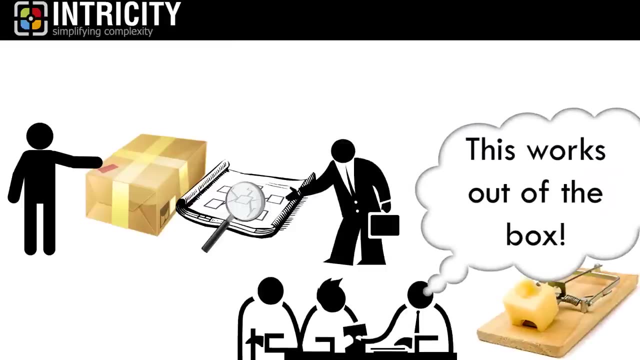 don't realize The amount of effort that you would take in vetting a packaged data model to make sure that it fits your business is nearly the same level of effort to go ahead and design one specifically for your business. However, this is an easy trap to fall into, because data models 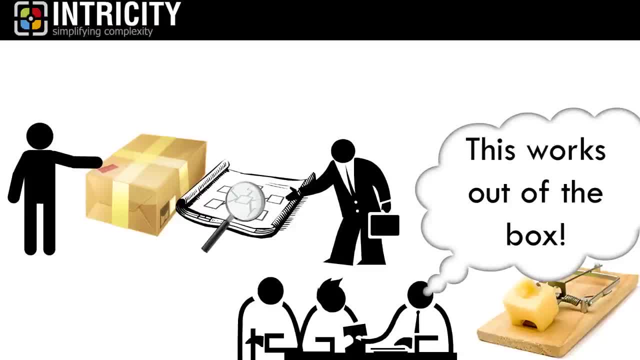 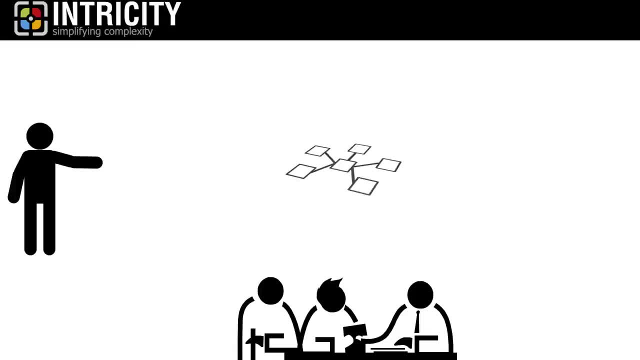 appear to do more than they actually do, especially to business people. The first thing to understand is that a data model is just a shell. A data model without populated data isn't much more than a drawing. The real example is a data model with less populated data. The real example is a data model. 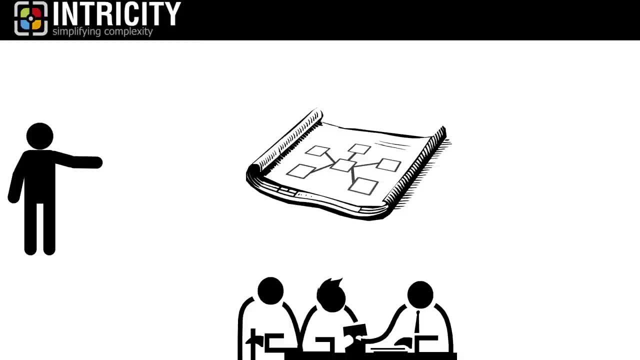 with less populated data. This is a data model without populated data. This is a data model with Expense, and heavy lifting in a data warehouse project is not in the design of the model, but rather populating that model with data from your source systems. 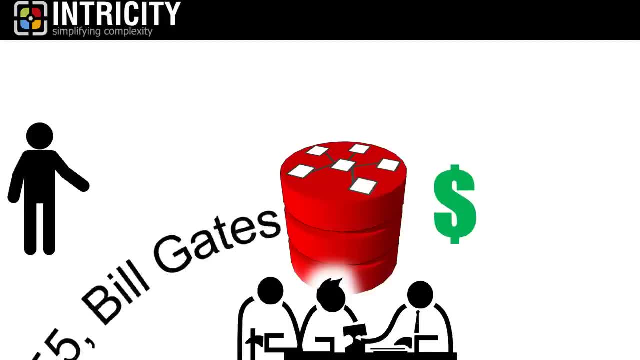 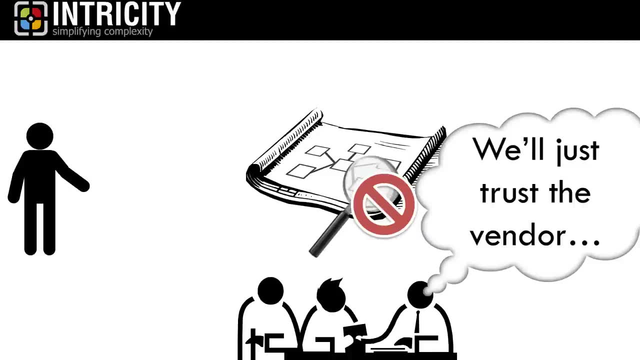 And that is where the big money is spent to create a data warehouse. Now, some organizations don't even vet packaged data models, assuming that they're well positioned out of the box, But they're usually in for a huge shock once all the reporting and analytics go live. 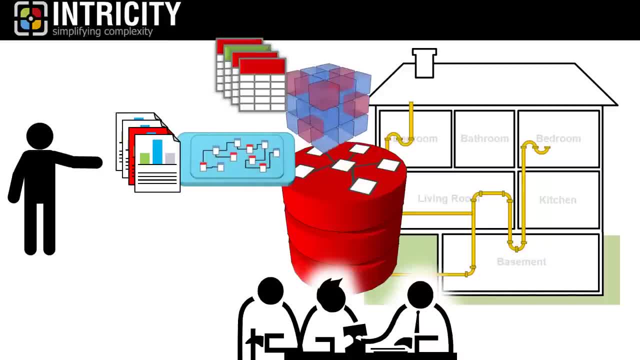 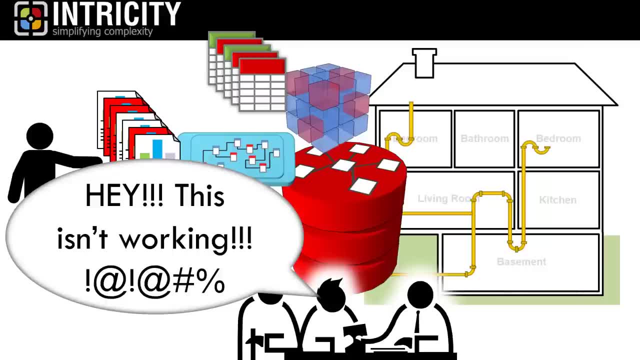 They often find that the logic does not mirror their internal practices and rules. Additionally, they find entire dimensions not being represented, Like our example with the home fixing. the problem is an expensive rip and replace process because the entire house around the pipes is already built. 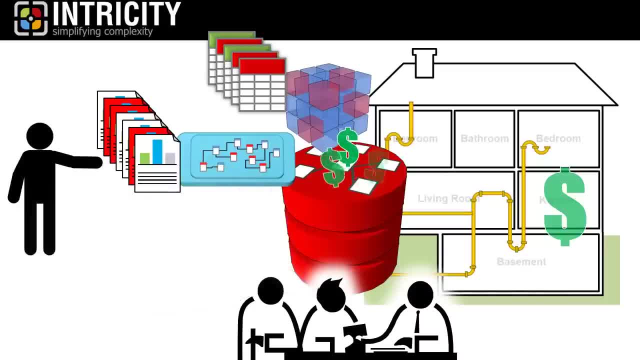 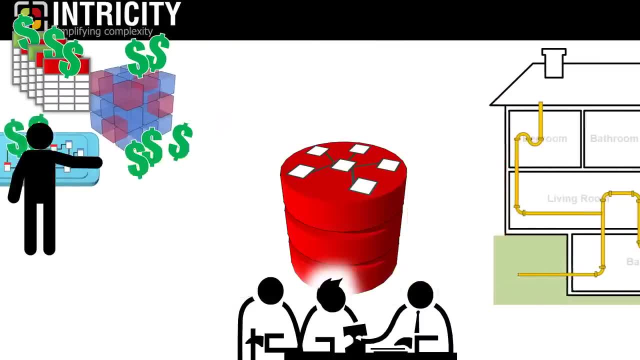 The same is true for the data warehouse. The ETL staging data model and reports are all in place and now need a major rebuild. If you're going to use a packaged data model, at the very least you should vet it completely before deploying it to your business.